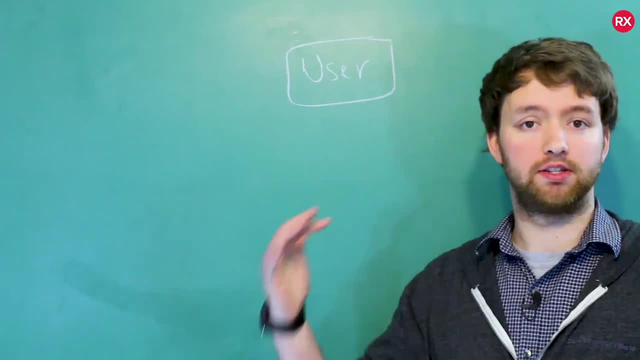 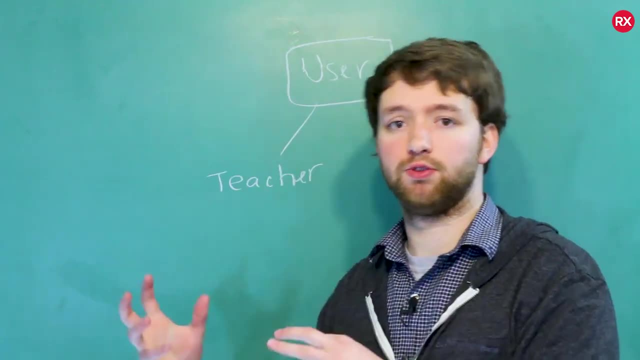 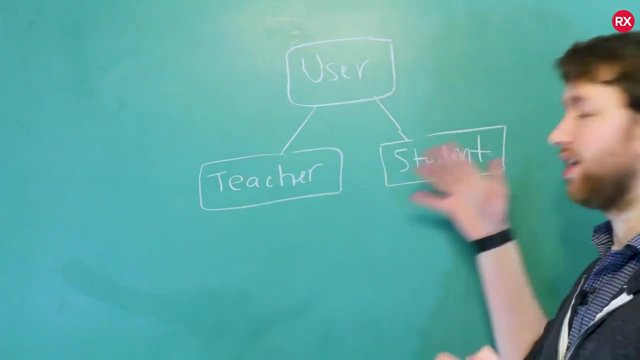 want to contain about a particular user, And then we might have what are known as subclasses that inherit from this user class. Let's say we're making an application for teachers and students. You might have a teacher class and you might have a student class. Now, if you think about it, 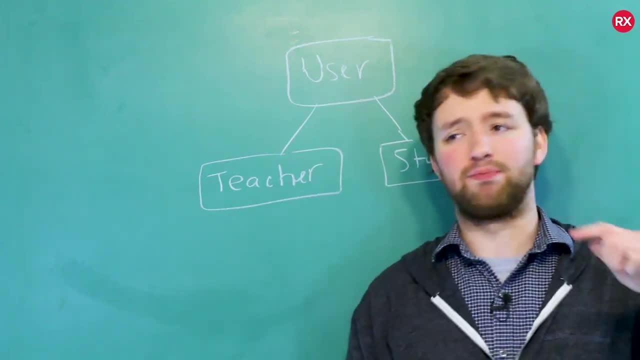 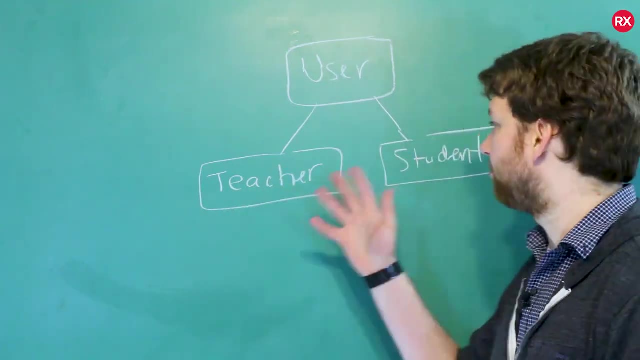 teachers and students have a lot in common: They both got names, they're both humans and so forth. So why have duplicate content in both of these classes If you need to describe teachers and students separately, in separate classes, but the majority of the content of the class is shared. 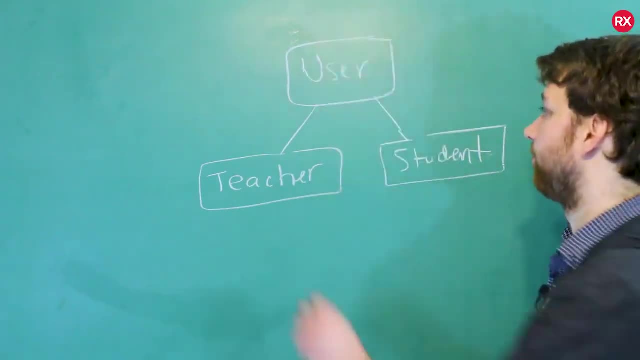 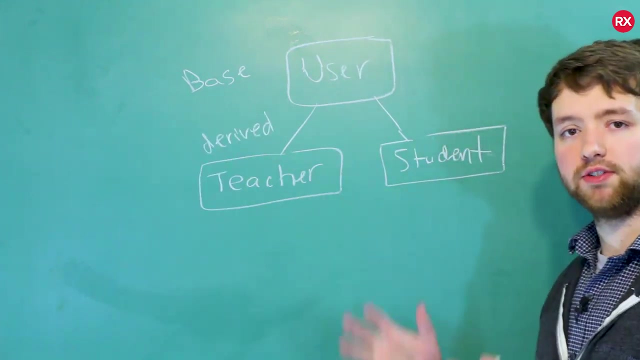 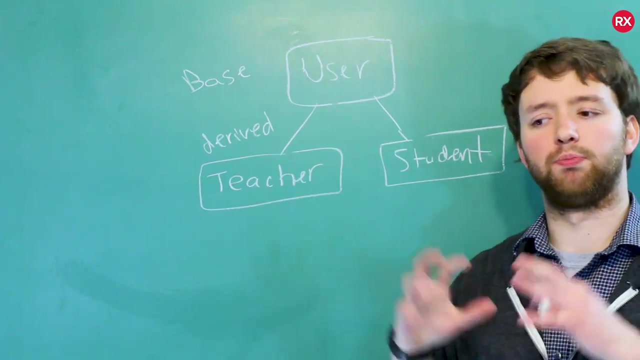 amongst them. you can put it in what's known as the base class. So here is the base and here are the subclasses or, more appropriately, derived classes. So this is a pretty good example, but you might also have animal and then dog and cat, because those have a lot in common, But they're 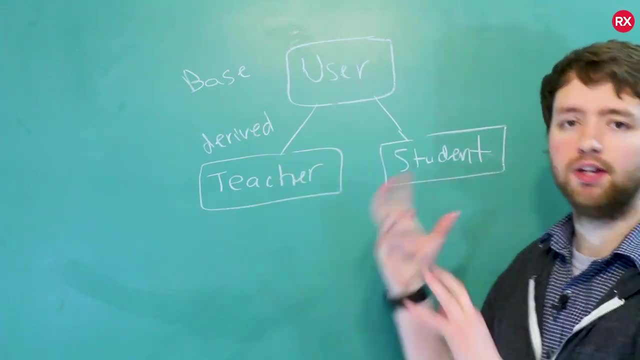 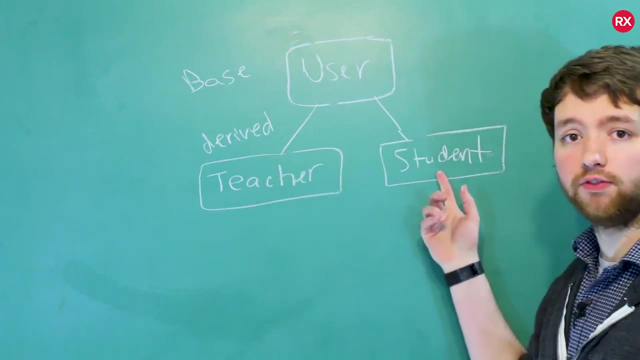 probably distinct enough that it would be appropriate to have them in the same class. It depends on the application. You might also have media file and then video file, photo file and then maybe a text graphic file, Like when you type on like a video editor or 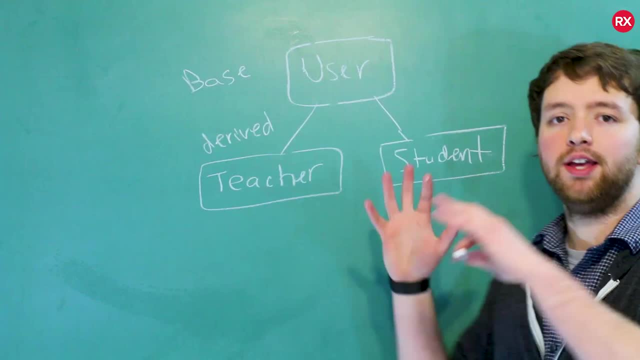 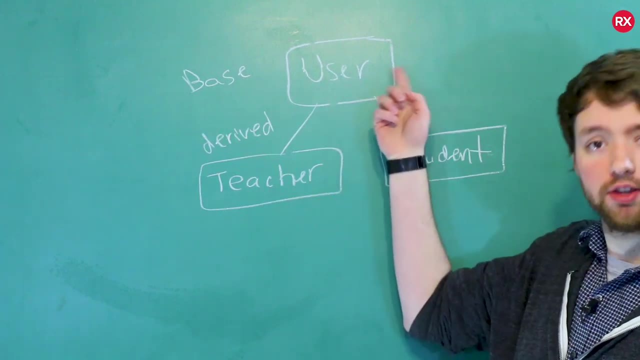 whatever The actual entities that we're describing is less important, and the concept behind it is what is more important. Basically, the teacher is going to get all of the stuff that's in the user and the student is going to get all the stuff from the user as well. 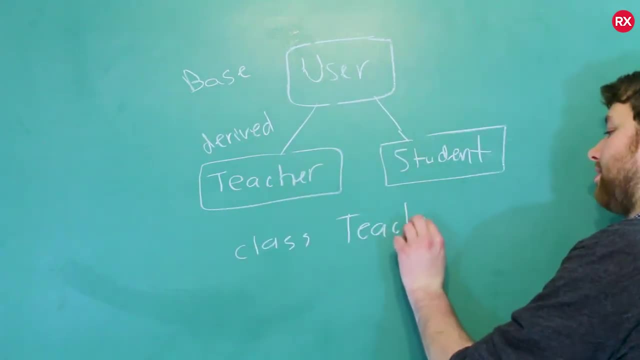 When you define the teacher, it's going to look like this: You're going to say class teacher and you're going to put a colon and then say public user. So that is how you establish that connection. You're going to inherit the stuff from user. Now the public there you don't really need 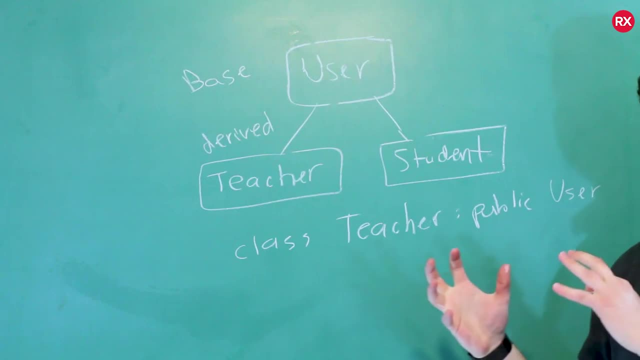 to worry about that. but you can put different access modifiers there if you want to basically change the way the members are inherited, Change the access of the members. I'm going to keep them all a default. so to do that, we're going to put public. 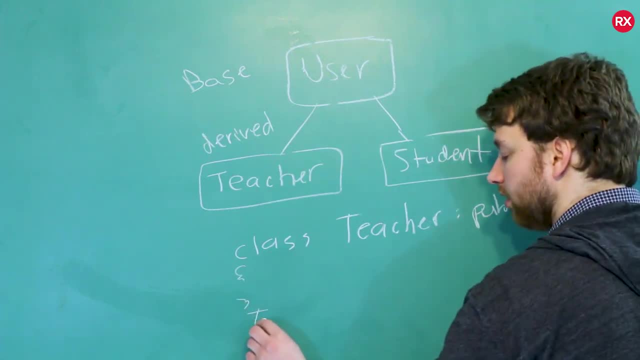 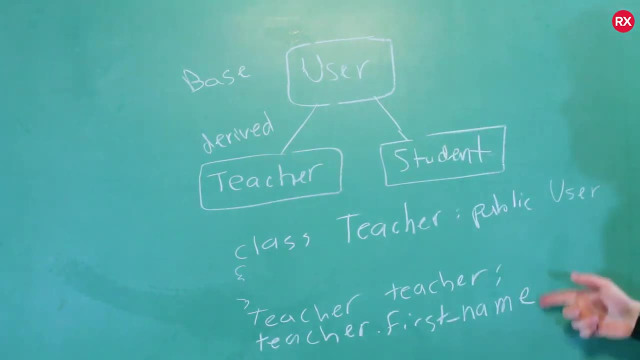 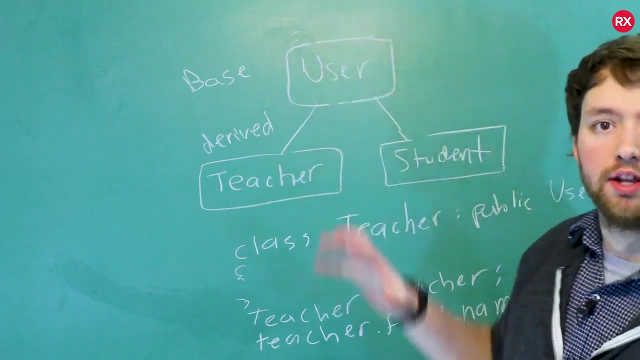 So, even if this class is empty, we can still create a teacher and call things on this teacher, So we could say teacherfirstName. That's because this first name is probably defined in this user class. You can do the same thing for student: Get the first name from the user. Now, why would you do? 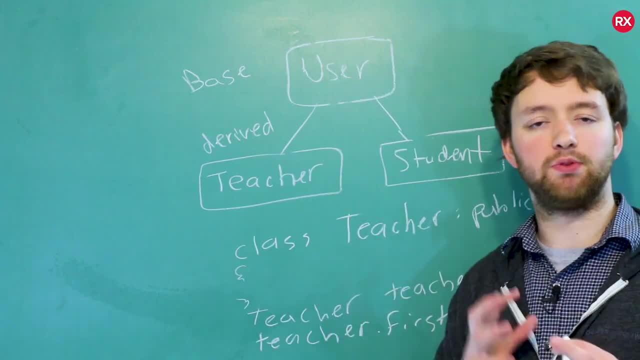 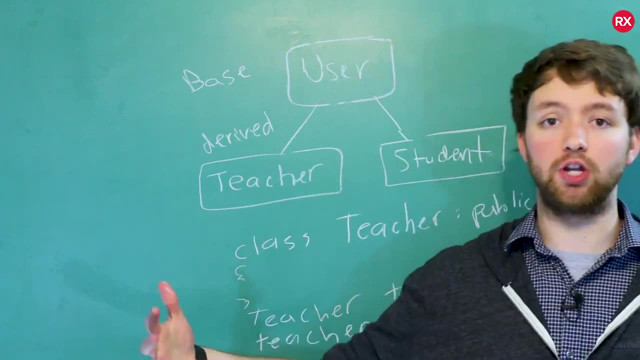 this. Why not just make them both users? Well, probably because there's some distinguishing factor between teachers and students. For example, inside of the teachers class, you can have a collection of classes teaching. Inside of the student class, you could have a data member such as the student's major, if this was a 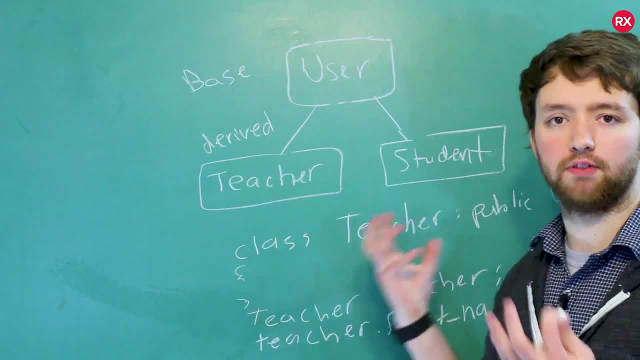 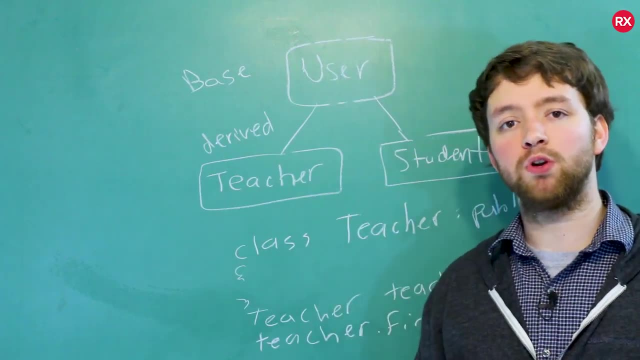 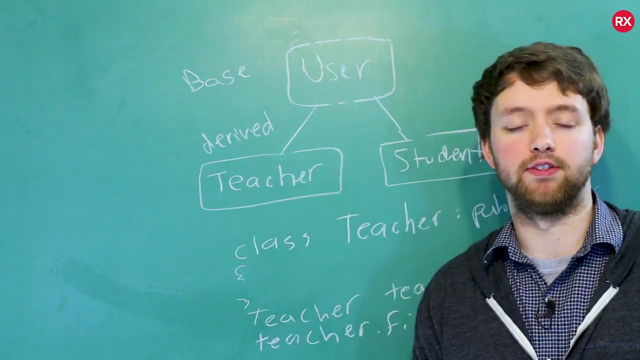 college. You can distinguish these entities but share a lot of common things by deriving from a base class. So that is the concept of inheritance. Now polymorphism is hand in hand, very similar in nature, because it kind of comes from inheritance, The idea behind polymorphism. you can treat a 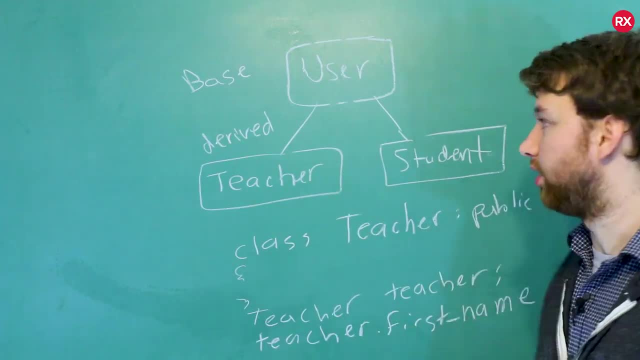 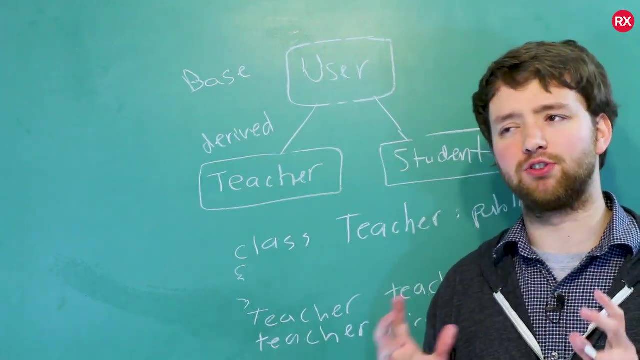 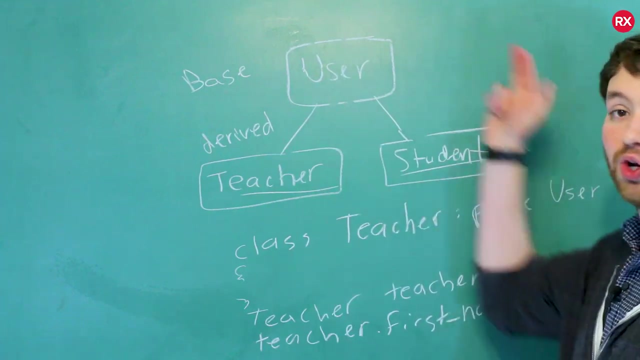 teacher as a teacher, or you can treat the teacher as a user, Because the teacher is both a teacher and a user. It's kind of confusing in nature and when I say it out loud I kind of sound like a psychopath. That's because a teacher qualifies as a user and a student qualifies as a user as well. 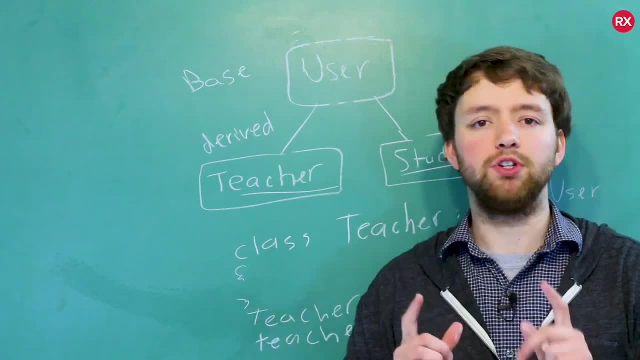 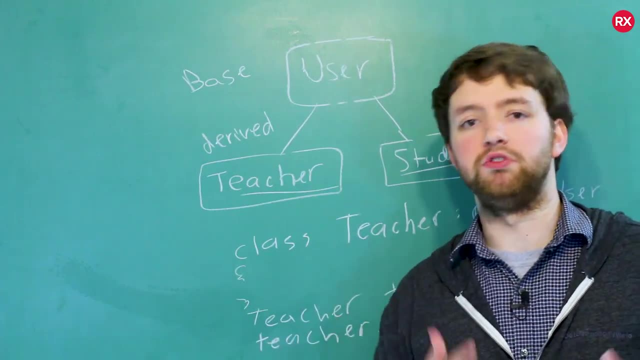 Now this seems like such a simple observation, but it's really useful because we can actually talk to all the derived classes as if they are users and they will do the appropriate thing. So, for example, we could say: users, get to work, and what's going to happen? 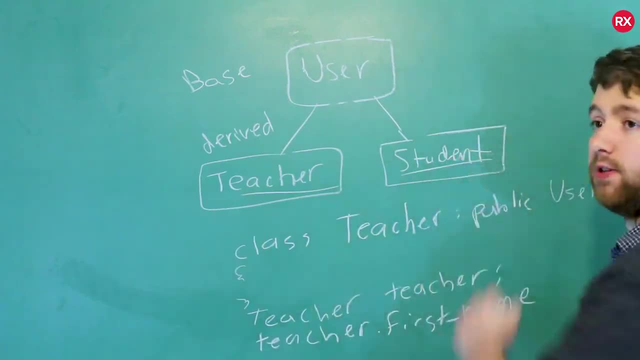 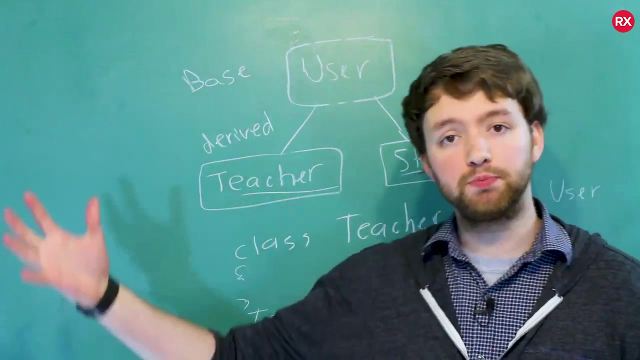 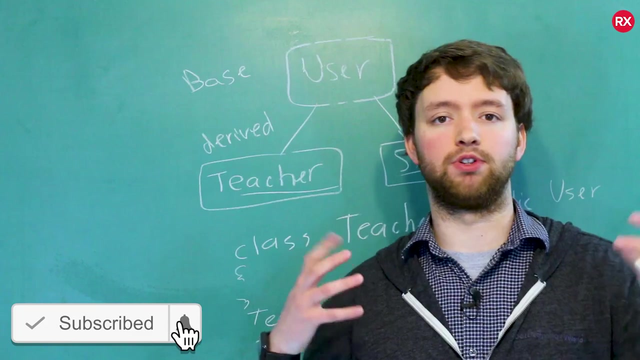 Is the teachers are going to go teach stuff and the students are going to start studying. Now C++ has something known as multiple inheritance, meaning a class can derive from multiple classes. This is not something you can do in like C sharp, for example. C sharp has the concept of interfaces, which is another common object oriented programming. 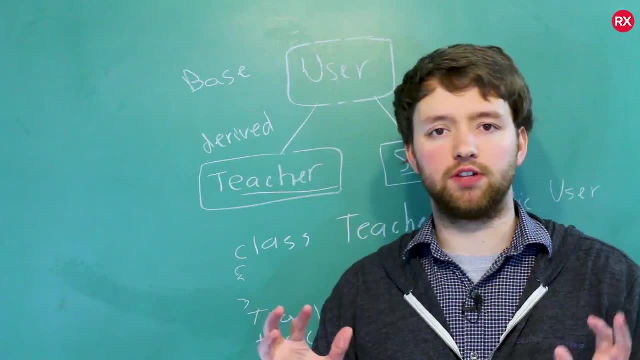 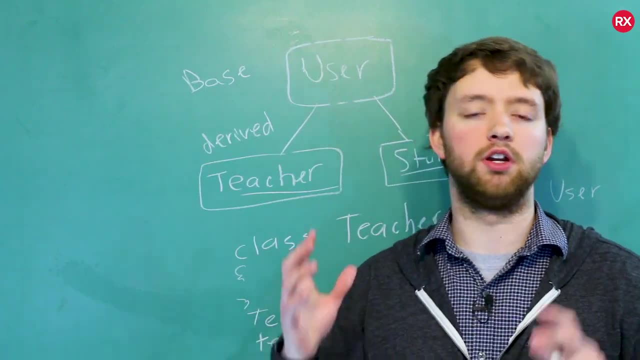 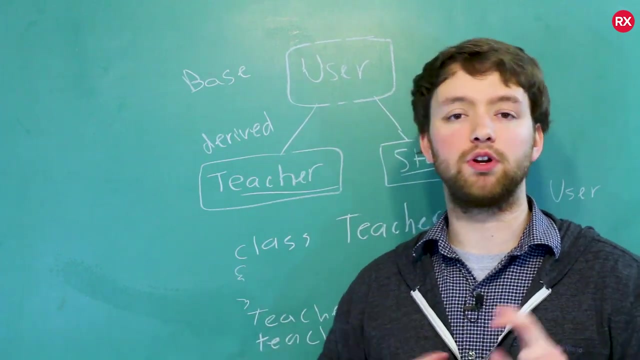 technique. But don't worry about all those differences. the main thing you need to understand is the concepts of inheritance and polymorphism. Once you got that down, you can go ahead and go learn about the different techniques for implementing object oriented programming in the different programming languages, Because this is just like the basics. we're not going to. 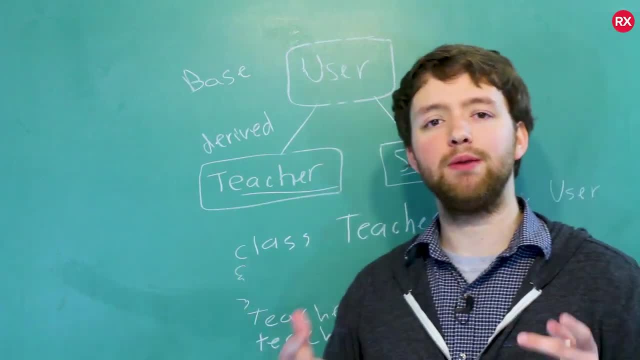 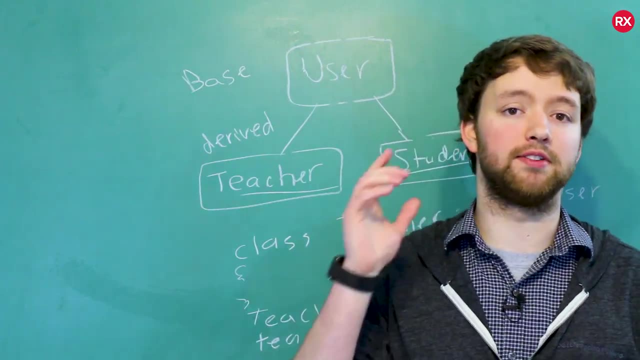 get into that. We're just going to inherit from one class and, you know, maybe, if you guys are good, I'll do a special video on multiple inheritance later on. So that's all I got for you guys to understand the concepts of inheritance and polymorphism. Hopefully that was helpful. 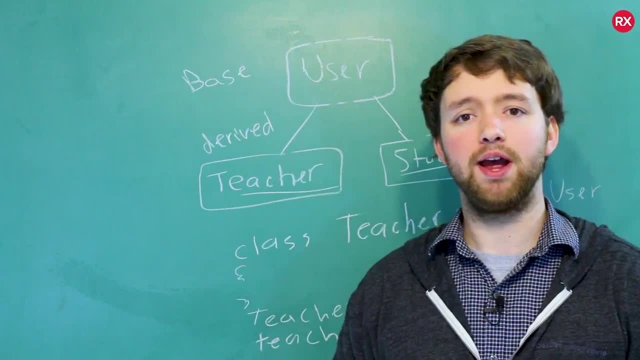 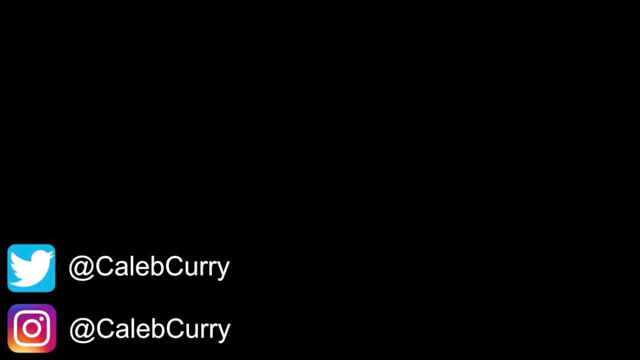 and now let's go do some practice exercises. Alright, peace out and be sure to subscribe Outro Music.